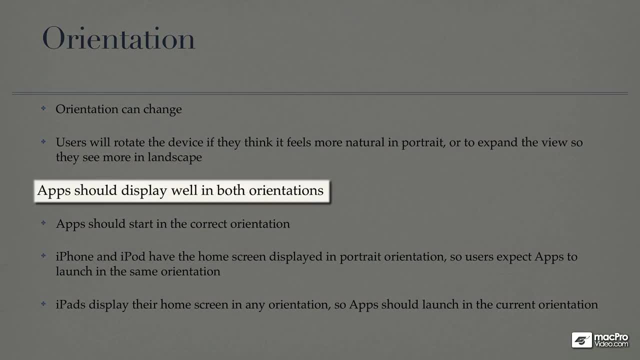 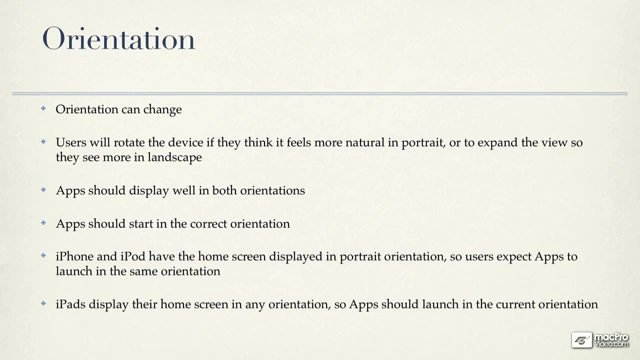 will do so as well. Your app should display well in both orientations And it should also start in the correct orientation. iPhone and iPod have the home screen displayed in portrait orientation, So before they actually launch an app they see all the icons lined up properly in portrait, But if they turn, 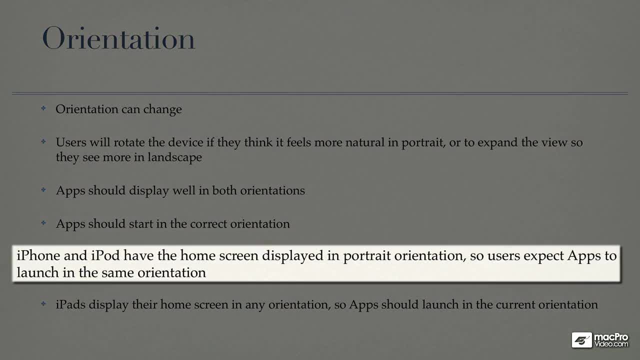 it sideways. in landscape it does not display correctly. It is still in portrait orientation, So if they launch an app, they expect it to appear in the same orientation as it was in portrait. iPads, however, can display their home screen in any orientation, So if they're in portrait, 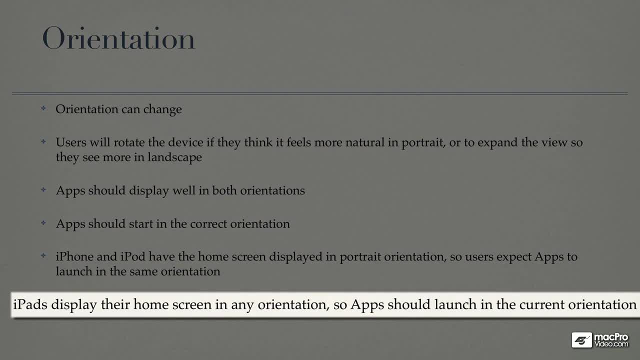 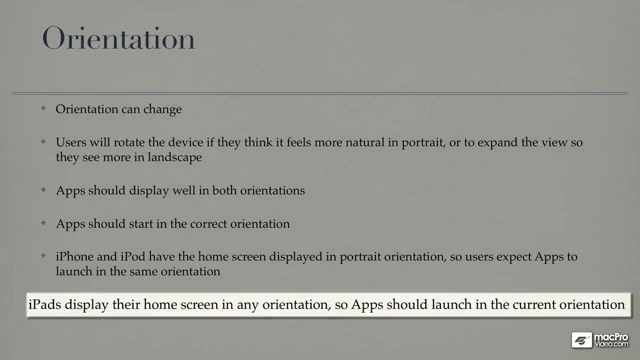 all the icons line up. If they turn it the other way- landscape- they all display correctly. They switch around, So when the app launches, it should launch in the same orientation automatically. The way users interact with the screen is with gestures, And the gestures that they 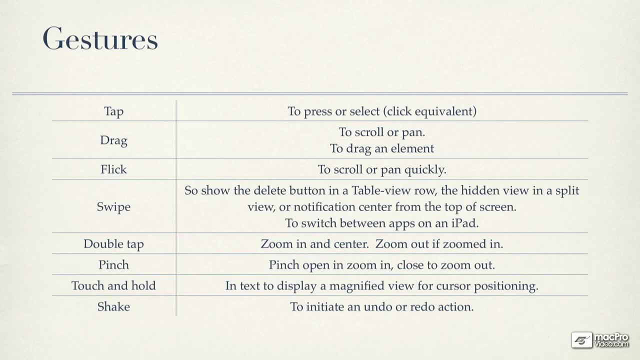 use in your app shouldn't confuse them. They should use the same standard ones to do standard actions. Or if you have to find custom ones, the custom ones should not be similar to the other ones. If we look at the typical ones, we've got tap, which is basically a click. We've got 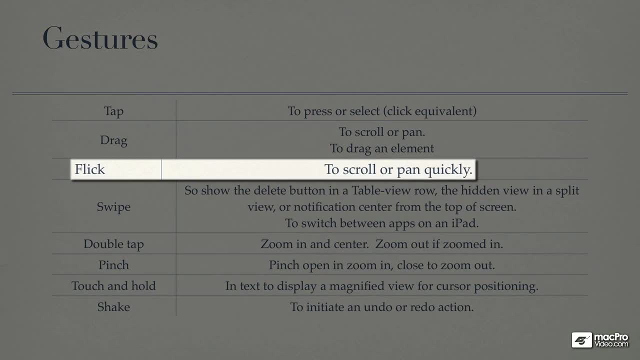 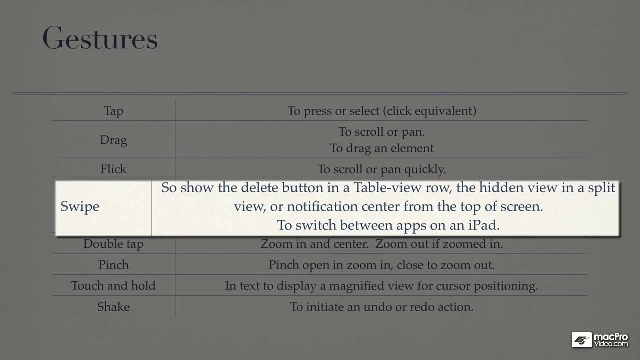 drag, which scrolls your pans, drags an element. Click is a quick scroll. You can tap to stop it. Swipe shows a delete button in a row, hidden view and a split view and the notification center from the top of the screen. 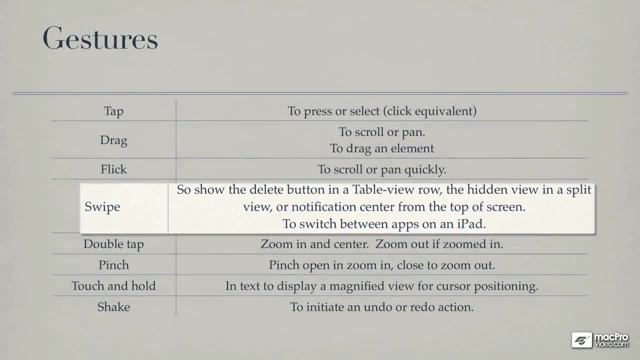 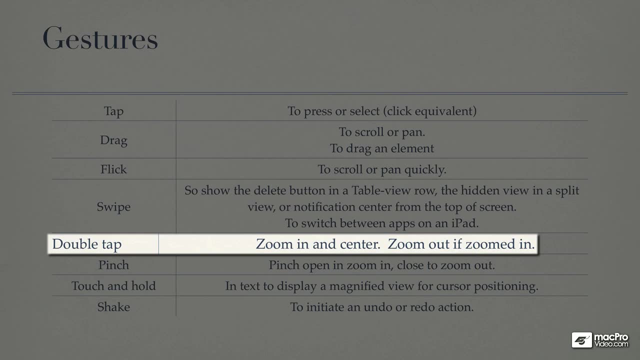 And a four-fingered swipe switches between apps. on an iPad, A double tap zooms- Zooms in and centers or zooms out. You can see this behavior in Safari on web pages with multiple columns. If you double tap on one of the columns, it expands to fill the screen. Double tapping: 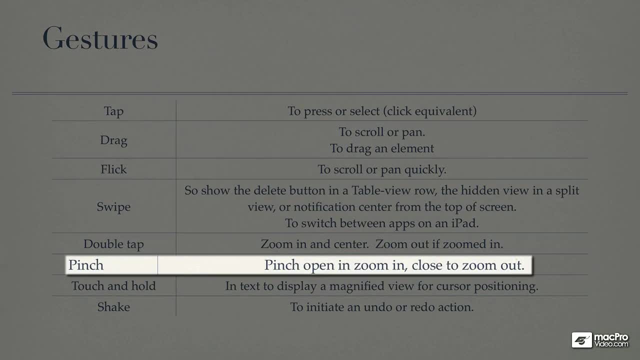 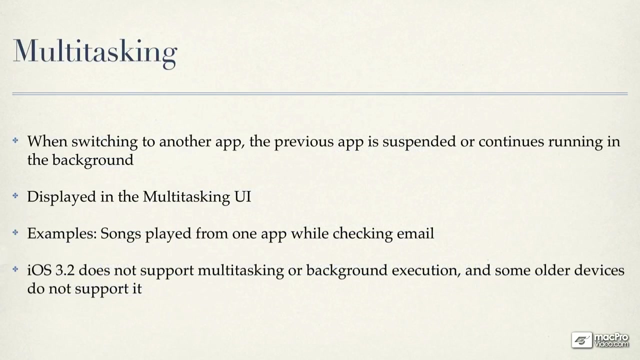 again shows the original view. Pinches, zoom in or zoom out, Touch and hold In a text area. it shows a magnified view so you can position the cursor, And a shake initiates an undo or redo action. We've also got multitasking. 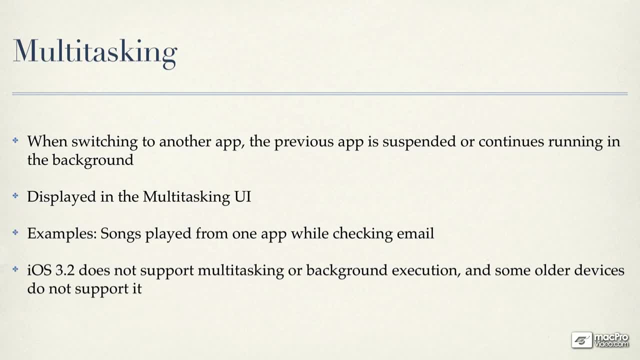 So if you receive a phone call while using an app, your app can choose to do one of several things: It may suspend or it may continue running it in the background. If you double click on the button at the bottom of the screen, you can see that the app is. 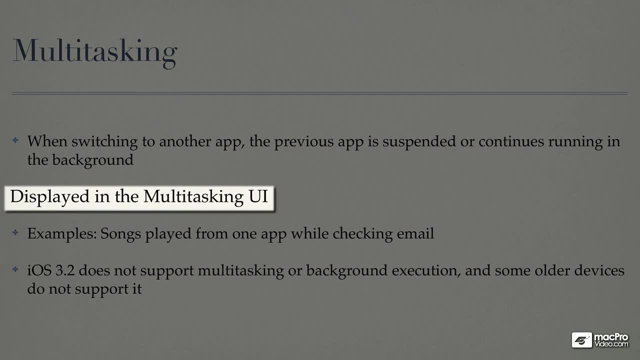 suspended. If you double click on the button at the bottom on an iPhone, you'll display the multitasking UI, And this is where you see apps that are suspended or running in the background. An example of this are songs that are played from one app while checking email. 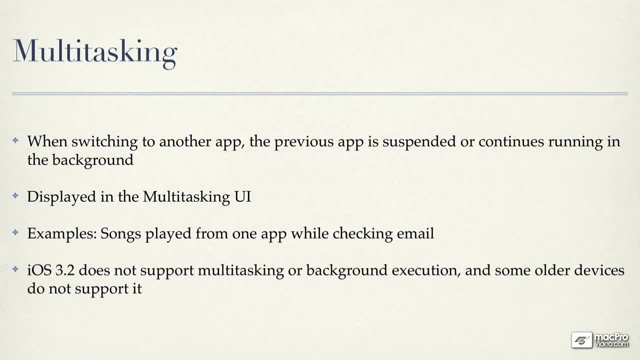 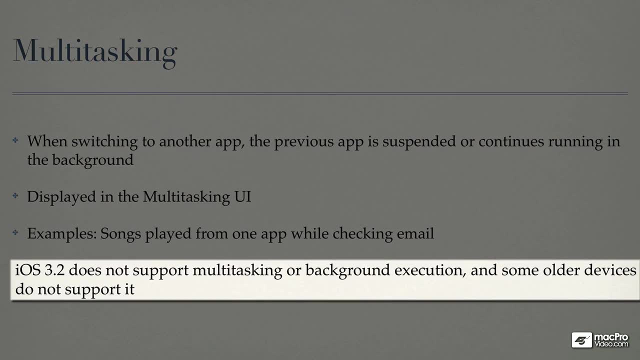 So you can still hear the song while you're using email. Certain versions of iOS- version 3.2 and earlier- don't support it. Some of the older devices also don't support it, So you have to be careful to make sure the device you're currently running on supports. 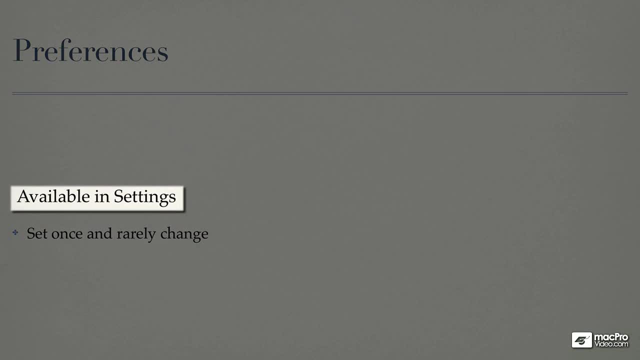 what you're trying to do. We've also got preferences which are available in settings. These are the ones that should only be set once or twice. They shouldn't be common ones that users are always changing. They're harder to get to. 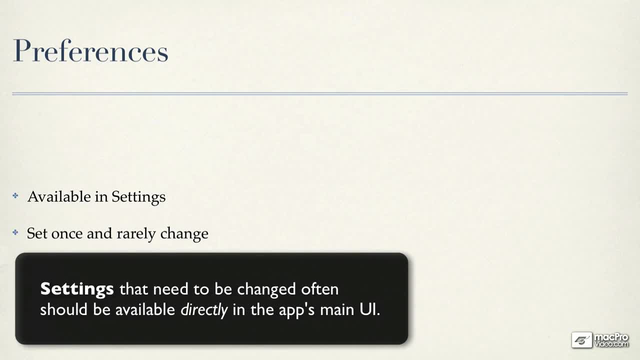 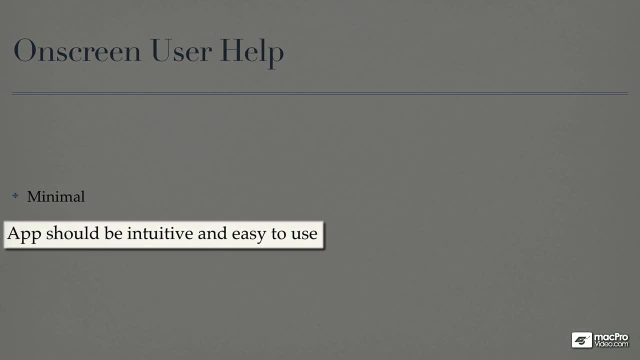 If you're going to have a setting that a user changes frequently, it should actually be in the app On screen user help. Your app should be minimal. It should be intuitive and easy to use. You shouldn't have a lot of extra stuff popping up. 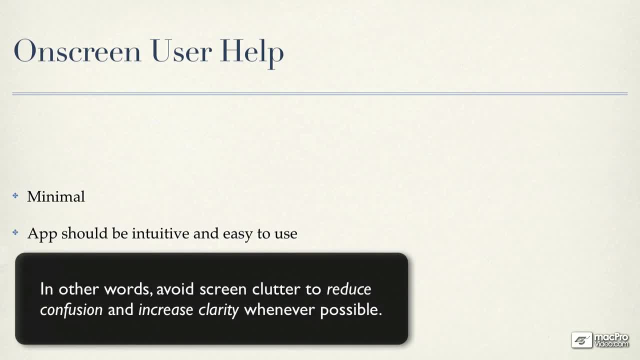 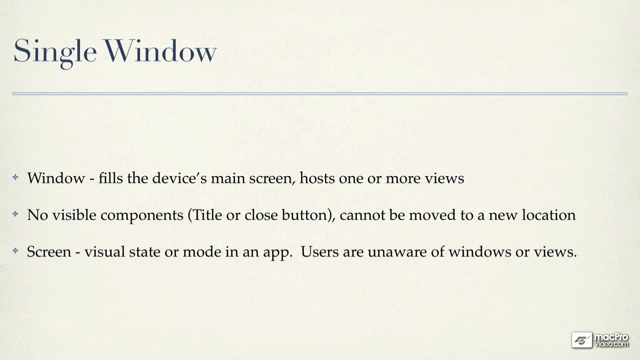 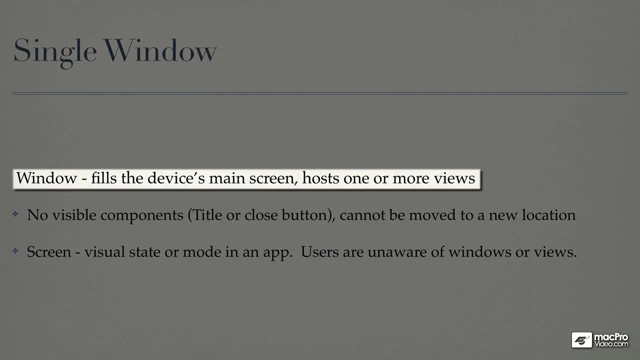 You should make sure Your buttons are named clearly and concisely so the user doesn't have to guess what they're trying to do. We have an area that the user is seeing. We've got a couple terms for this area. We can refer to the window, which is what the user doesn't see. 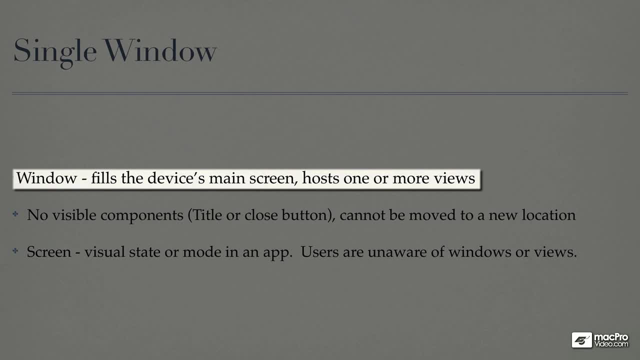 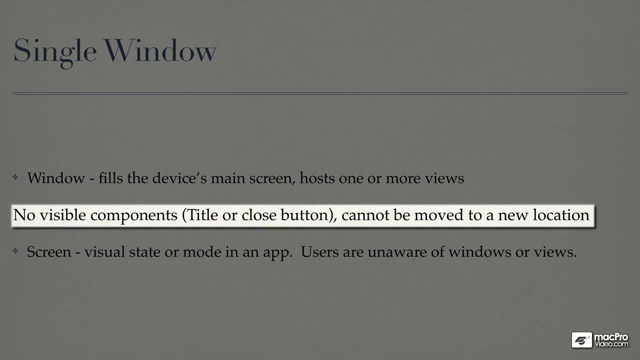 It's the area that hosts all the content that they would see, So it can host one or more views, and the views contain the content that the user interacts with. The window itself has no visible components. It doesn't even have a title or close button. 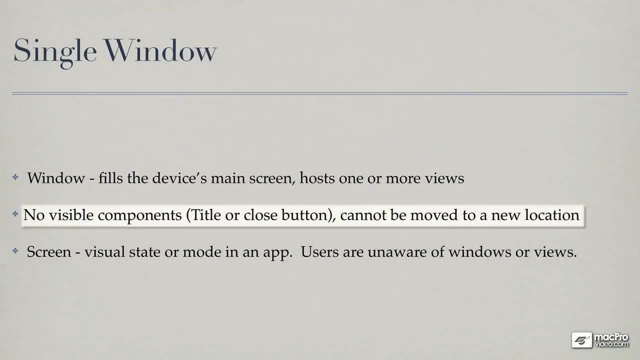 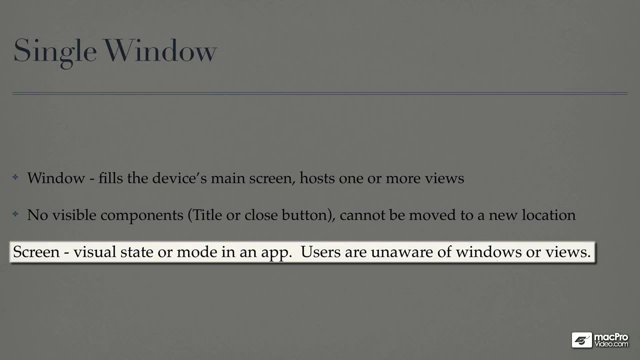 It can't be a new button. It moved to a new location and can't be resized. The screen is what the user considers. It's the visual state or mode of an app. They're unaware of windows or views. There could be multiple views in an iPad screen. 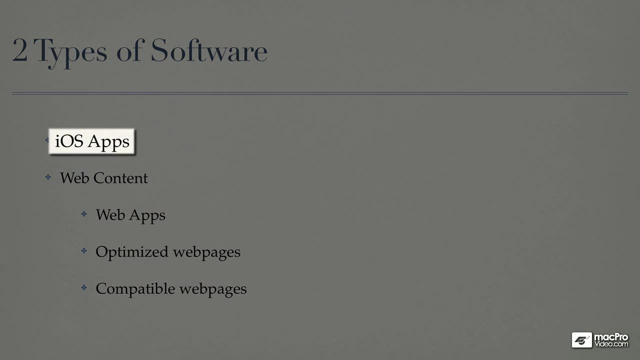 There's two types of software: iOS apps, which are the ones that we're developing with Xcode and with Objective-C. You've also got web content, so that would be HTML pages designed more or less for running on a mobile app. You have web apps.